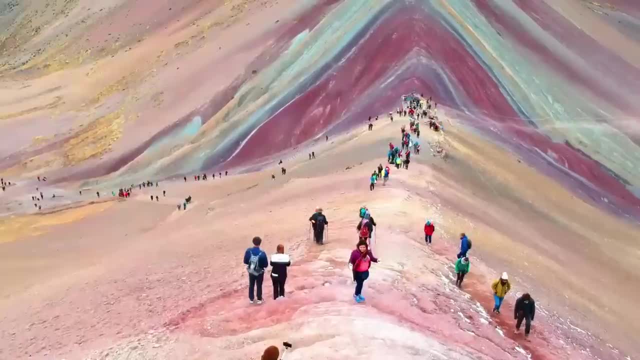 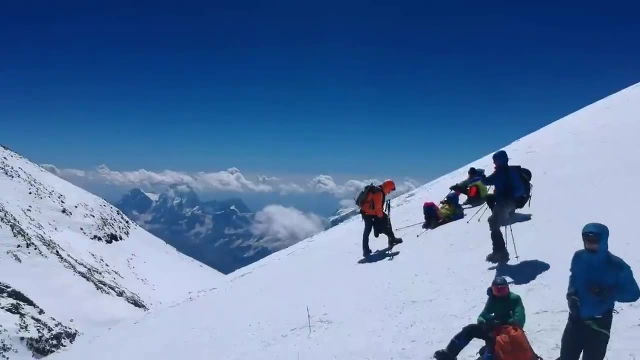 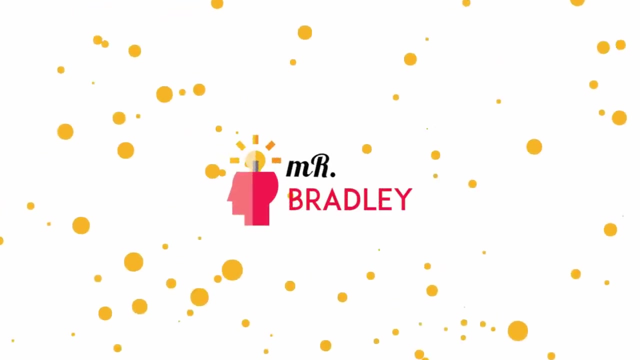 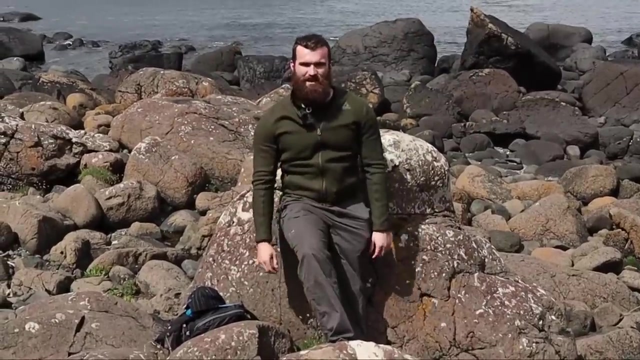 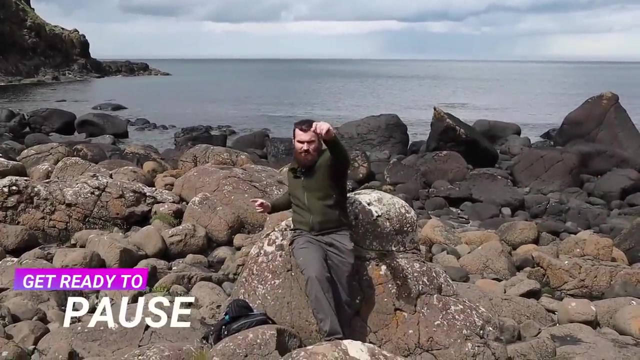 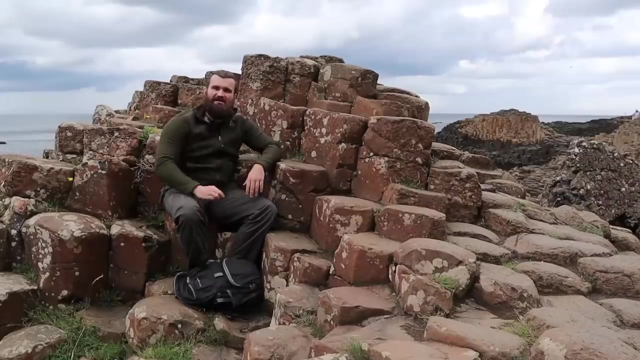 Hello everybody, it's me, Mr Bradley, and today we're learning about rocks. But before we begin, hit that subscribe button and get ready to do the starter questions on your screen right now. Rocks can be organized into three separate categories, depending on how they were formed. 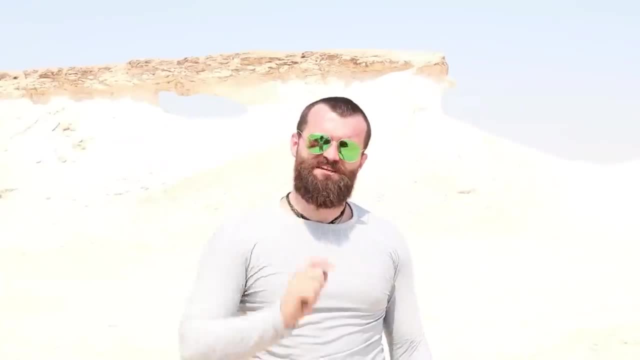 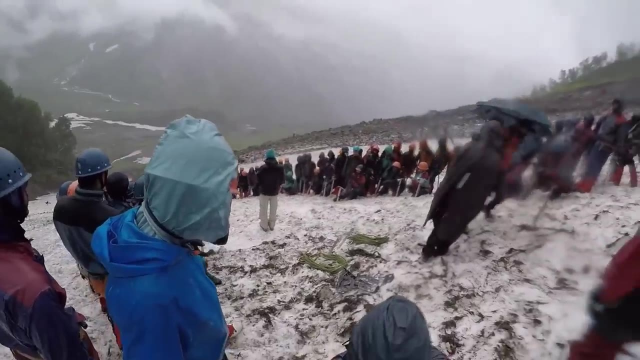 Igneous, metamorphic and sedimentary. The first kind of rock we're going to learn about is sedimentary rock. On top of mountains it can get pretty windy and rainy, And did you know that this wind and rain can chip away tiny pieces of rocks and dirt away from the mountain? 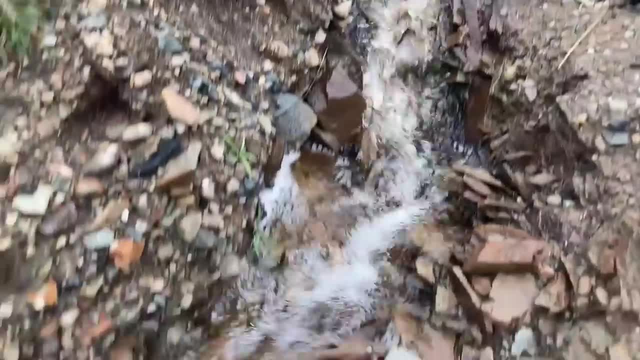 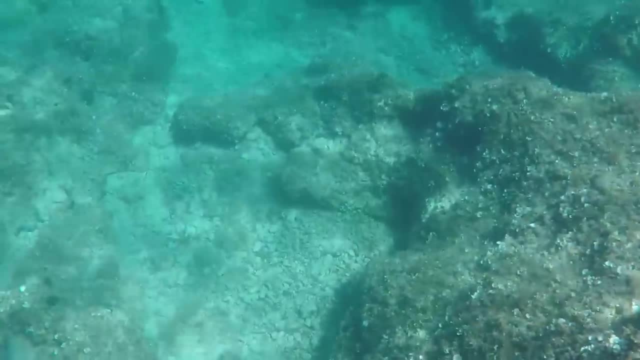 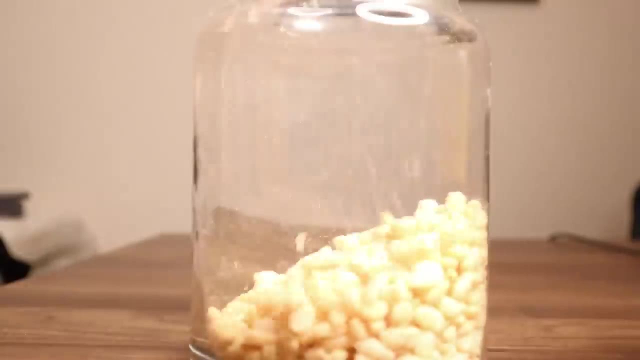 These tiny pieces of rocks and dirt are carried by water down streams to rivers, finally reaching oceans and lakes where they sink down to the bottom. We call these tiny rocks and dirt that sink down to the bottom sediment. Over time, more rocks and dirt sink on top of them. 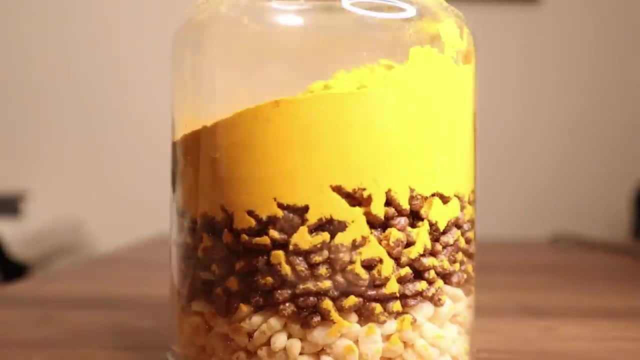 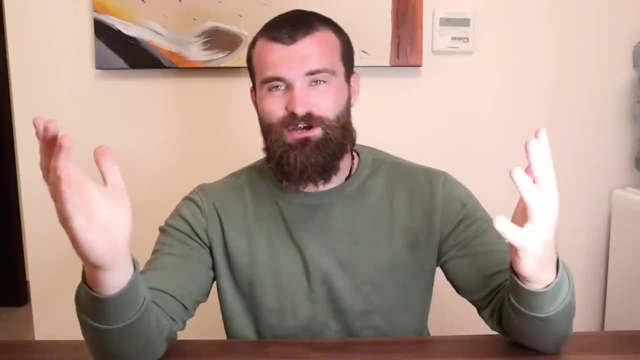 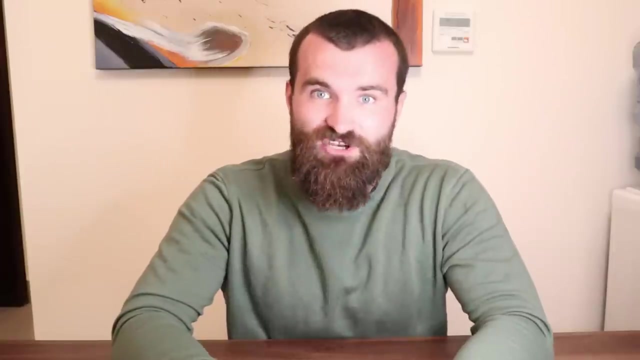 then more sink on top of them, then more on top of them. After a long time, zillion, jillion, dillion, cotillion times later, things start to get heavy for the rocks and dirt at the very bottom. These layers are squeezed together harder and harder until eventually. 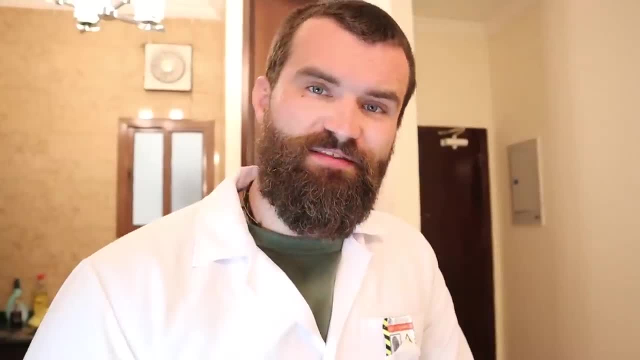 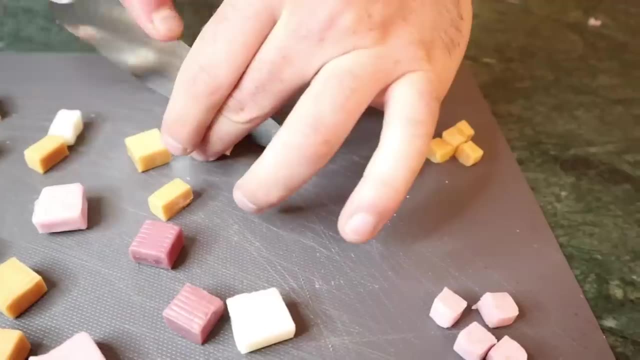 sedimentary rock is formed Now using these starbursts. I'm going to show you the rock cycle. So now I'm just going to cut up the starbursts into tiny little rocks, which we'll then use to make our sedimentary rock. 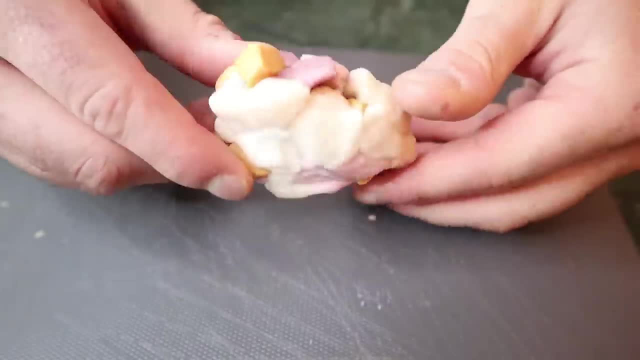 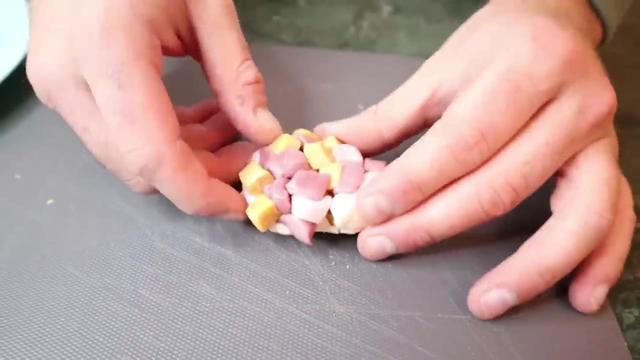 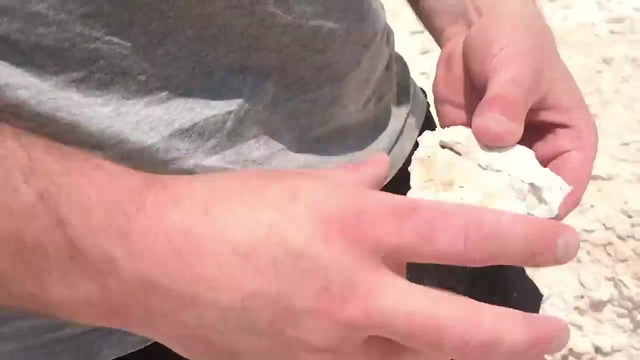 Okay, So our sedimentary rock is now being formed. This has been made of many smaller pieces of rocks and dirt all squeezed together to form one hard rock. Sometimes, these layers of rocks and dirt can be very clearly seen within the sedimentary rock formation, Although all rocks are pretty hard. 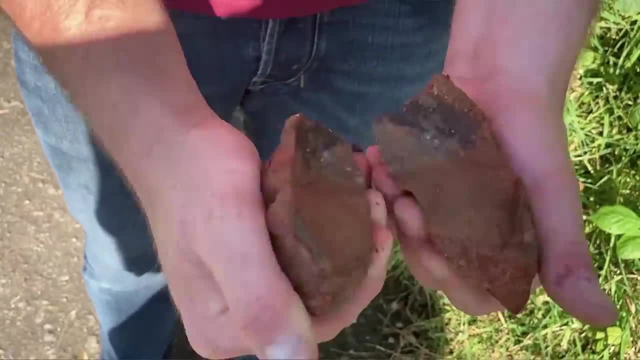 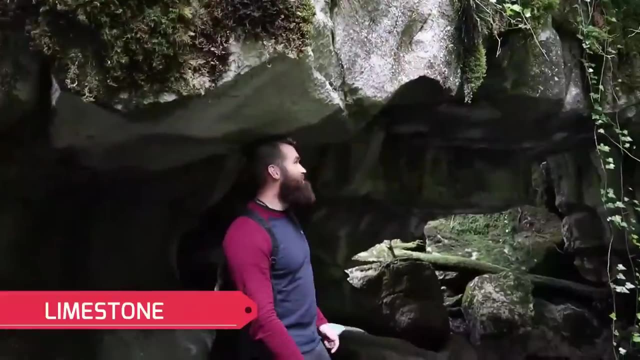 sedimentary rock is probably the weakest out of the three types of rocks. Examples of sedimentary rock include sandstone, mudstone, limestone, shale and even sandstone. The sedimentary rock is called coal, which we learned at a coal mine we visited here in Ireland. 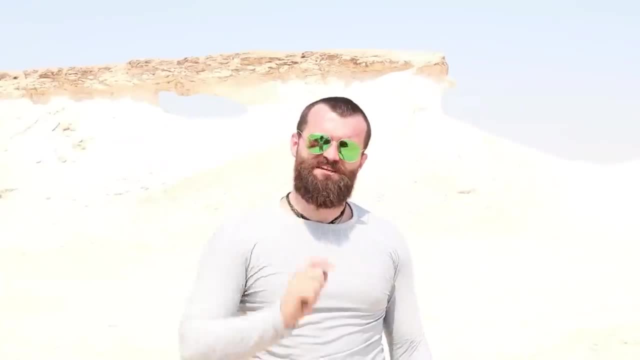 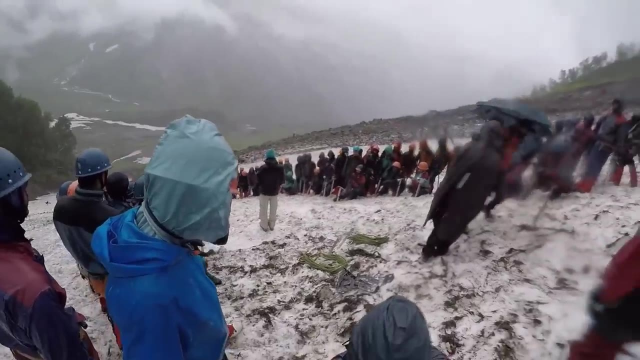 Igneous, metamorphic and sedimentary. The first kind of rock we're going to learn about is sedimentary rock. On top of mountains it can get pretty windy and rainy, And did you know that this wind and rain can chip away tiny pieces of rocks and dirt away from the mountain? 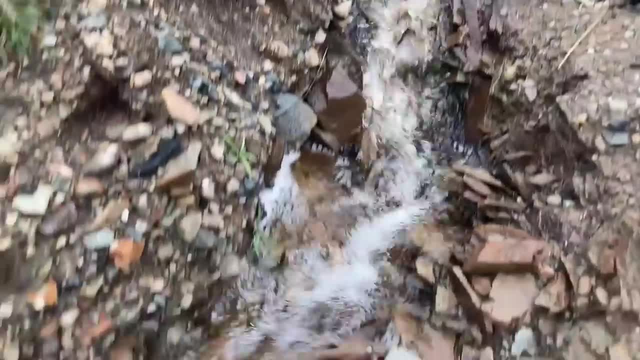 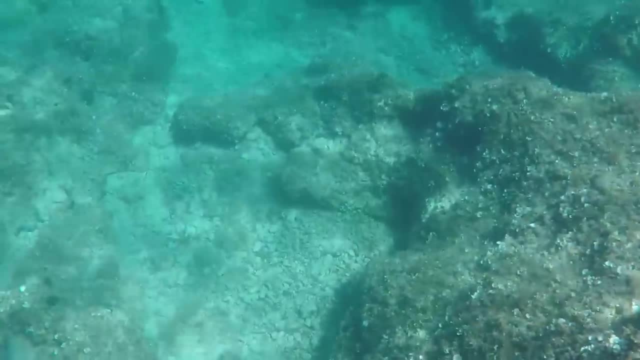 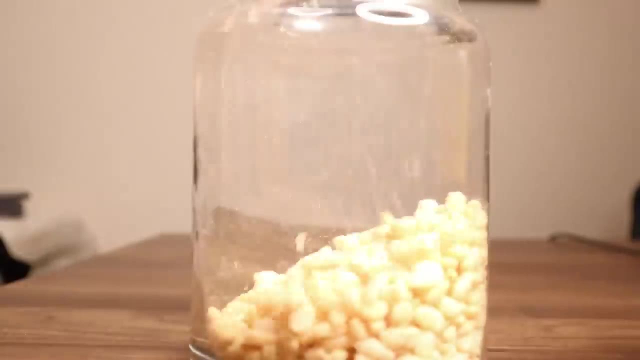 These tiny pieces of rocks and dirt are carried by water down streams to rivers, finally reaching oceans and lakes where they sink down to the bottom. We call these tiny rocks and dirt that sink down to the bottom sediment. Over time, more rocks and dirt sink on top of them. 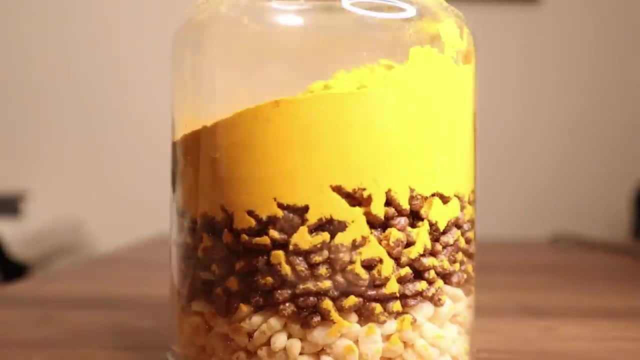 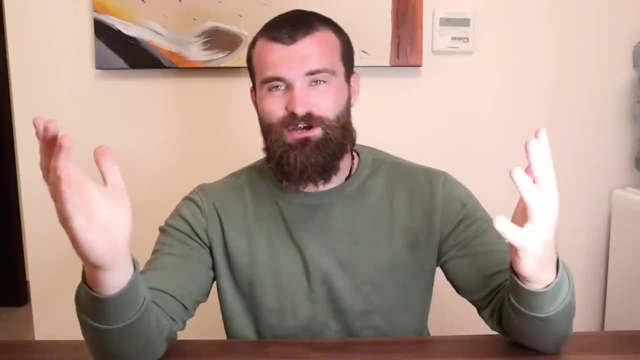 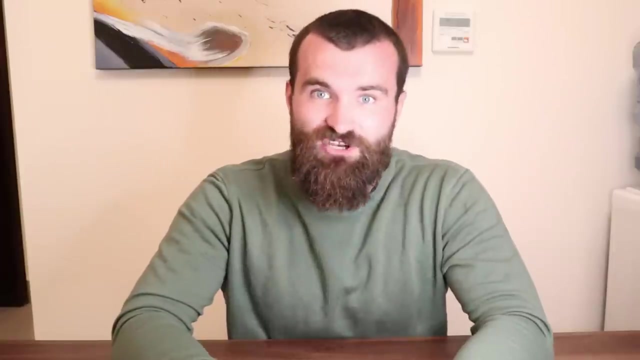 then more sink on top of them, then more on top of them. After a long time, zillion, jillion, dillion, cotillion times later, things start to get heavy for the rocks and dirt at the very bottom. These layers are squeezed together harder and harder until eventually. 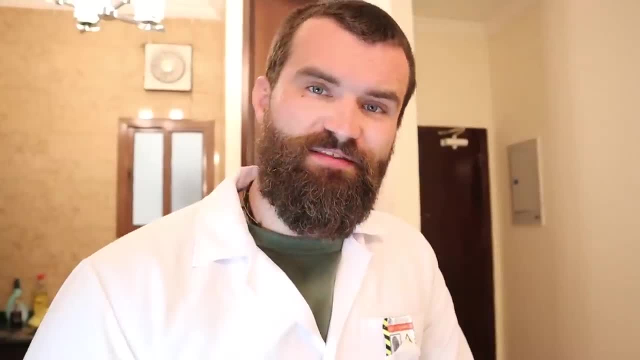 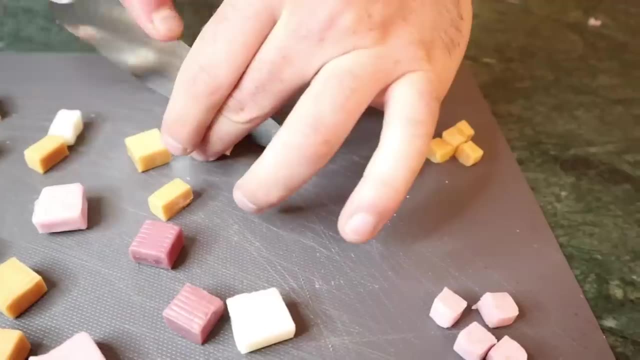 sedimentary rock is formed Now using these starbursts. I'm going to show you the rock cycle. So now I'm just going to cut up the starbursts into tiny little rocks, which we'll then use to make our sedimentary rock. 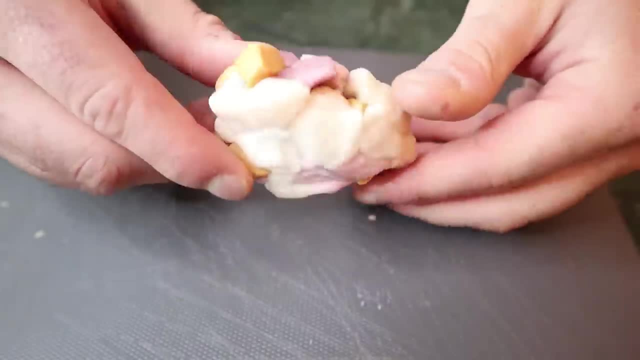 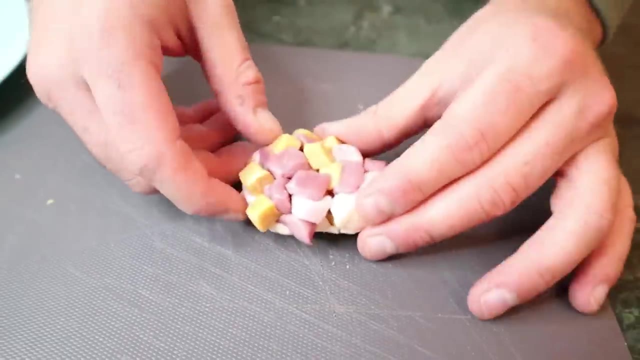 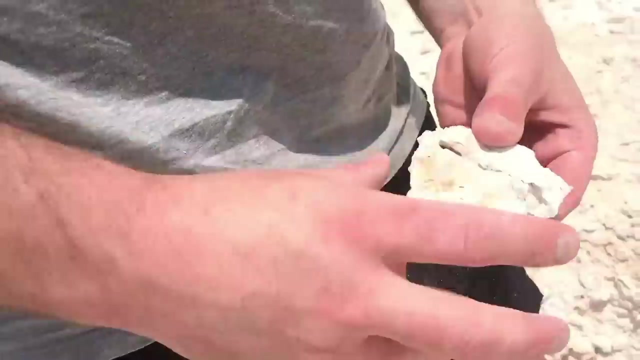 Okay, So our sedimentary rock is now being formed. This has been made of many smaller pieces of rocks and dirt all squeezed together to form one hard rock. Sometimes, these layers of rocks and dirt can be very clearly seen within the sedimentary rock formation, Although all rocks are pretty hard. 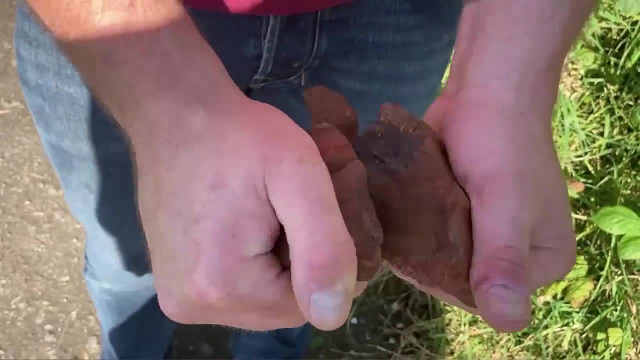 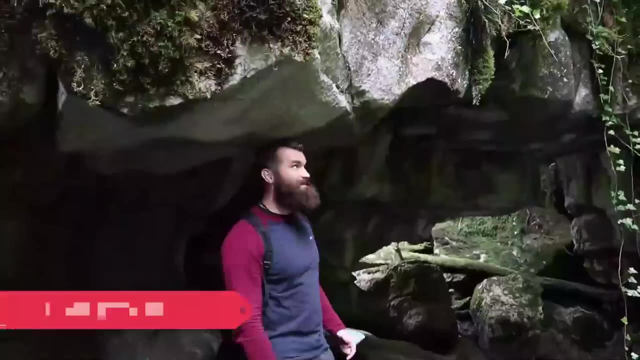 sedimentary rock is probably the weakest out of the three types of rocks. Examples of sedimentary rock include sandstone, mudstone, limestone shale and even sedimentary rock. In this video, I'm going to show you how to make a sedimentary rock using coal, which we learned at a coal mine we visited here in Ireland. 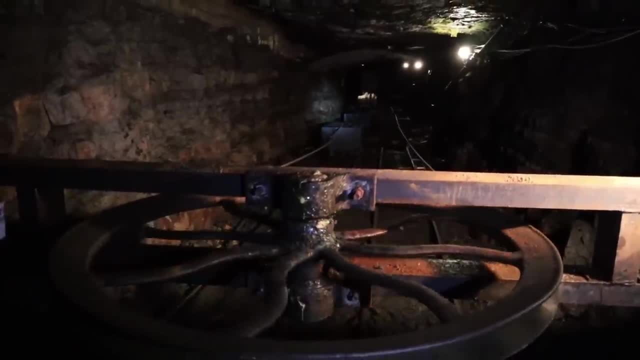 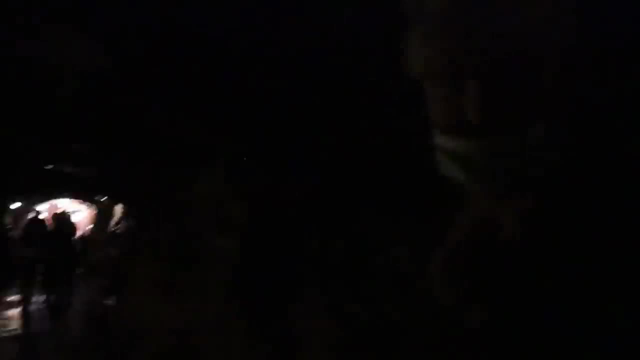 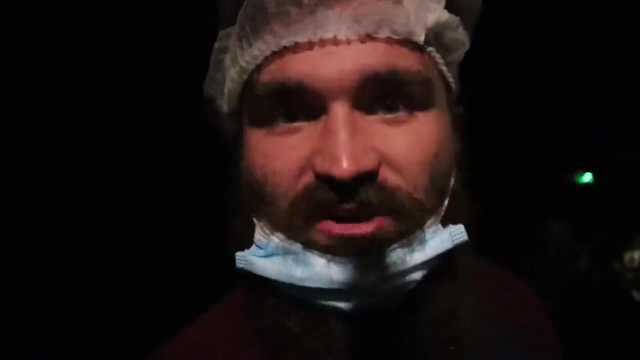 Hello, I'm here at Aurigna Mining Experience to learn about a very special kind of sedimentary rock called coal. So we're just here in Aurigna Mine deep, deep, deep onto the ground, And here is where coal is mined. Above me is layers and layers and layers of rock. 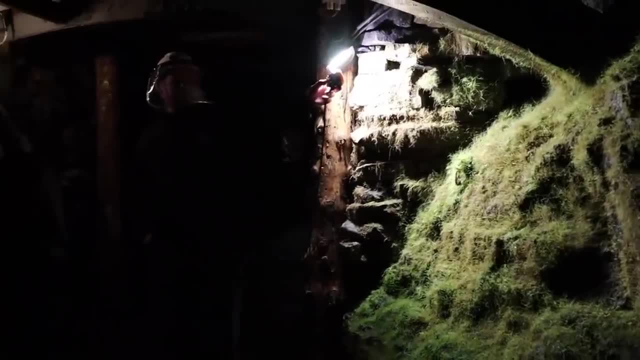 Very, very heavy. See how I can compress and squash down that sedimentary rock to make coal. Let's check out some incredible sedimentary rock to make coal. Let's check out some incredible sedimentary rock to make coal. Let's check out some incredible sedimentary rock to make coal. 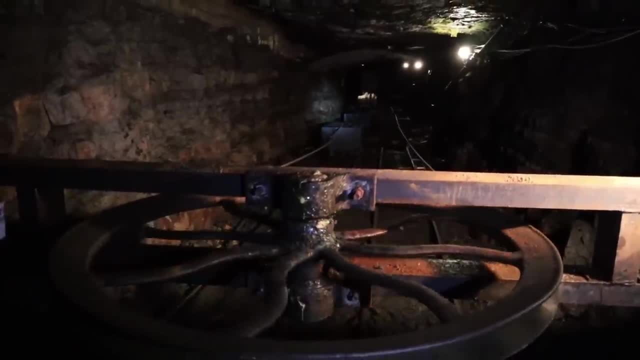 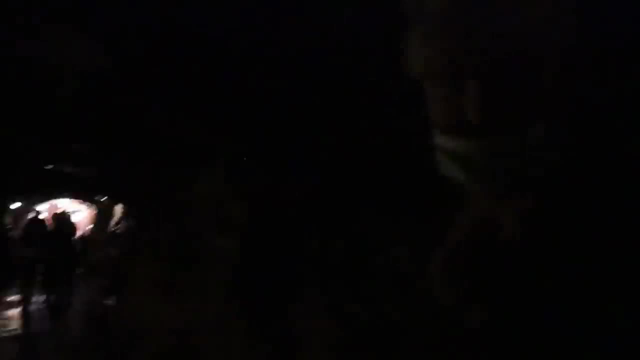 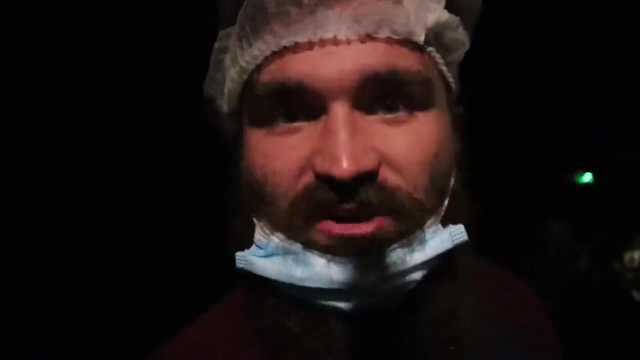 Hello, I'm here at Aurigna Mining Experience to learn about a very special kind of sedimentary rock called coal. So we're just here in Aurigna Mine deep, deep, deep onto the ground, And here is where coal is mined. Above me is layers and layers and layers of rock. 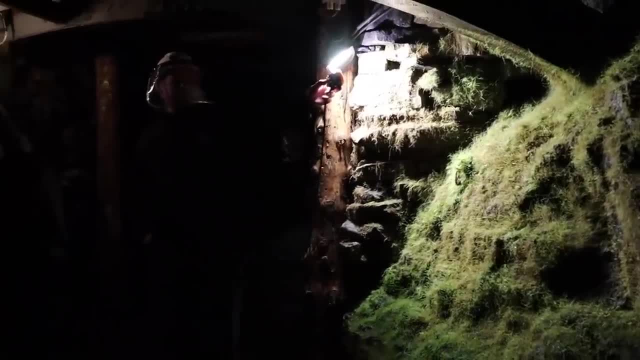 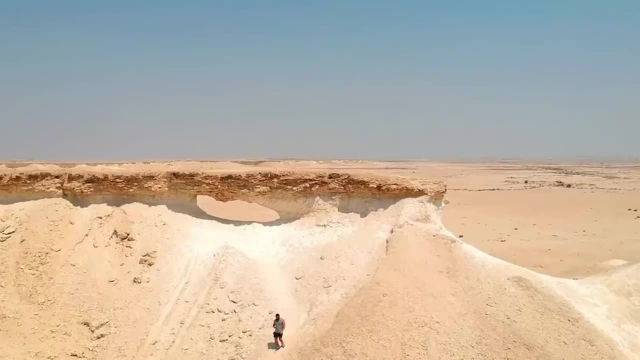 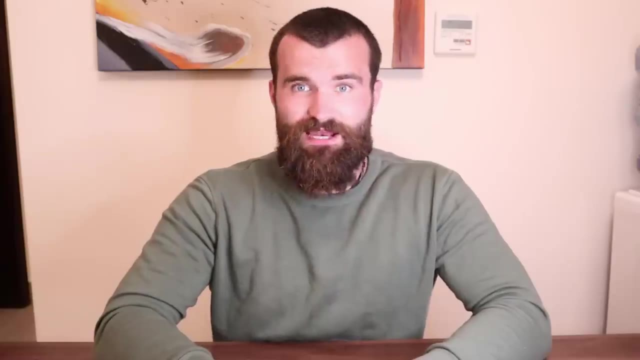 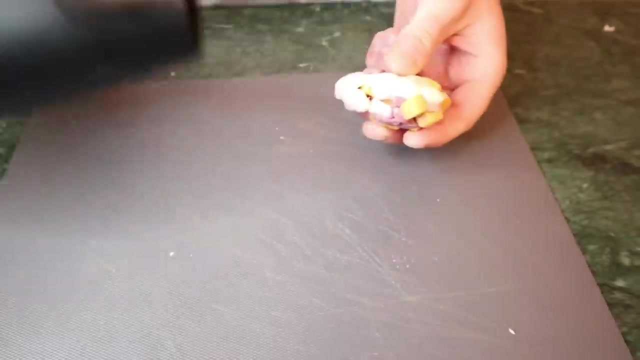 Let's check out some incredible sedimentary rock formations, And the next type of rock we're going to learn about is metamorphic rock. Sometimes, these layers of rocks and dirt deep underground become close to molten hot magma. To add a little bit of heat to this rock, I'm going to use a hair dryer. 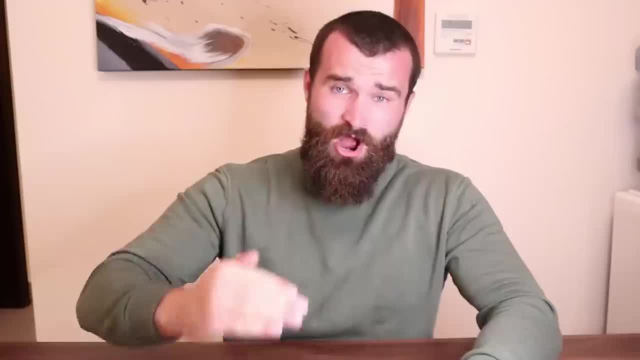 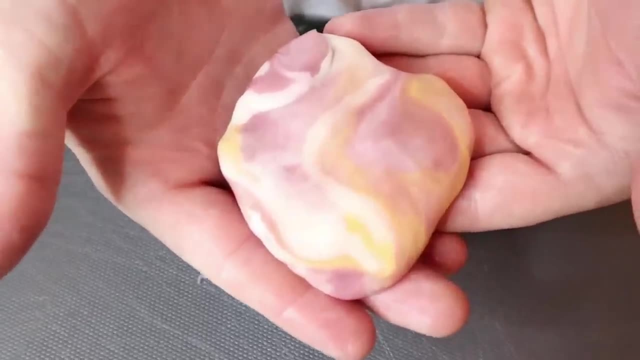 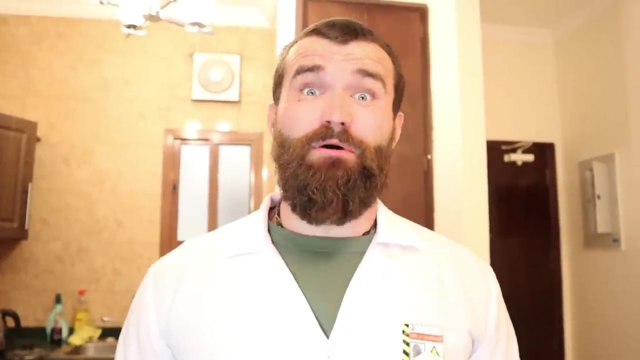 The heat of the magma, combined with the huge pressure of all of the layers of rocks above, can cause the rocks at the bottom to be chemically changed into metamorphic rock, But this also takes a super long time. Here's some footage of me climbing on metamorphic rock on a mountaineering course in India. 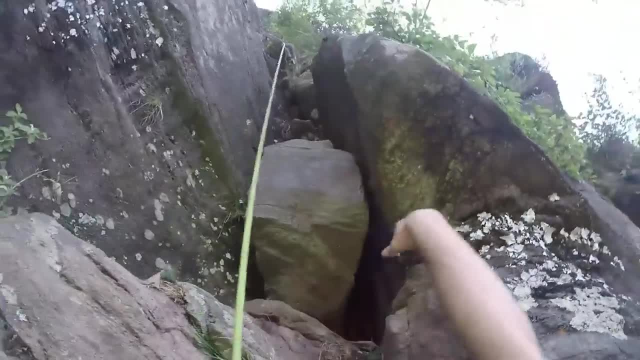 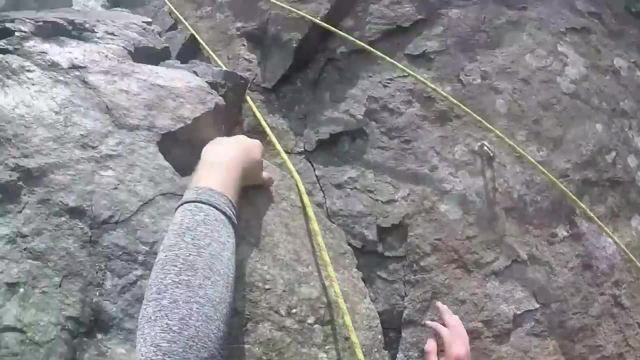 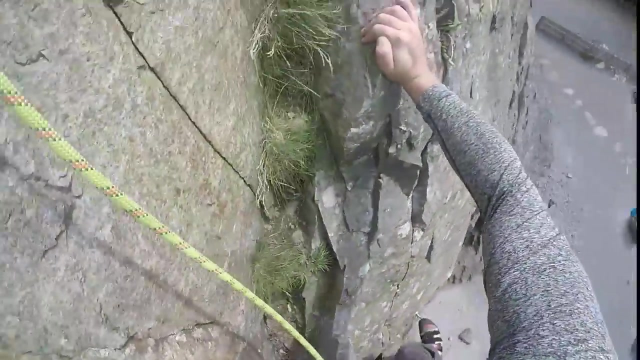 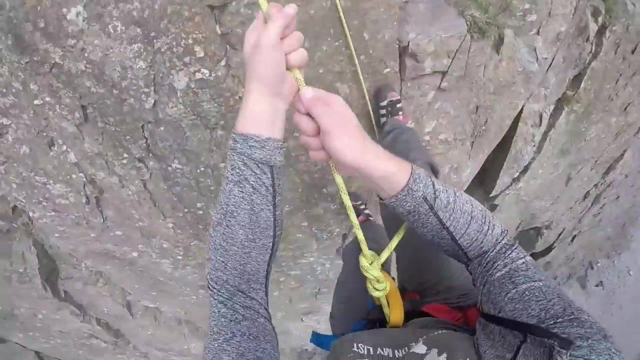 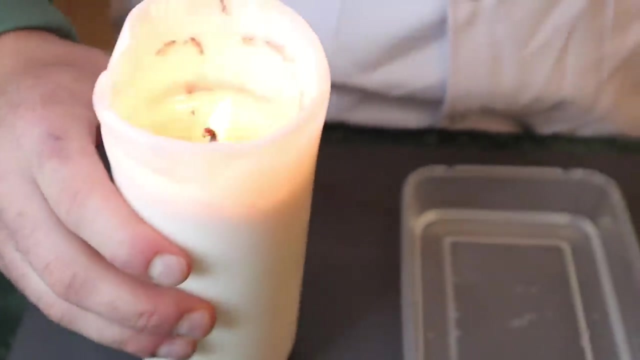 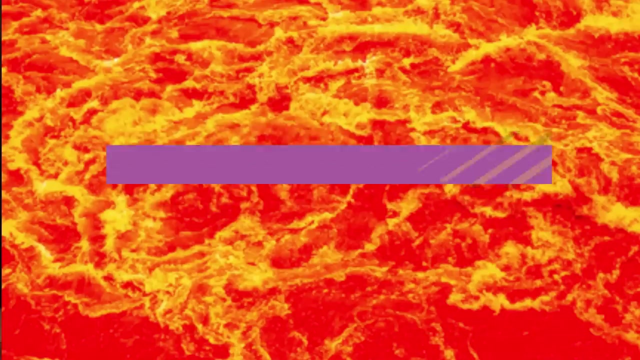 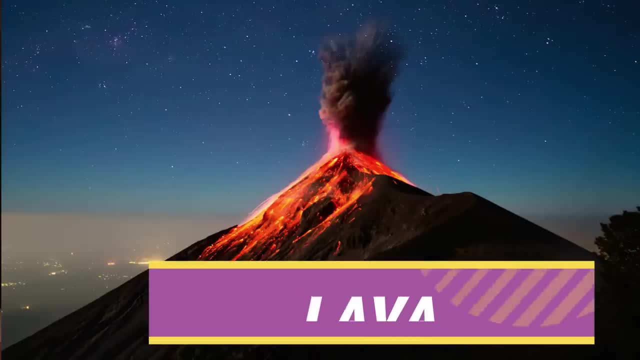 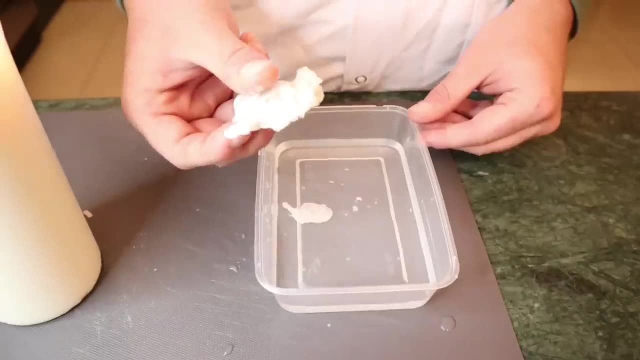 Molten rock that is underground is called magma, and molten rock that comes out of the ground is called lava. When the magma or lava cools down again, it hardens and forms igneous rock. Take a look at my starburst. When I heat them, they begin to melt and form molten rock. 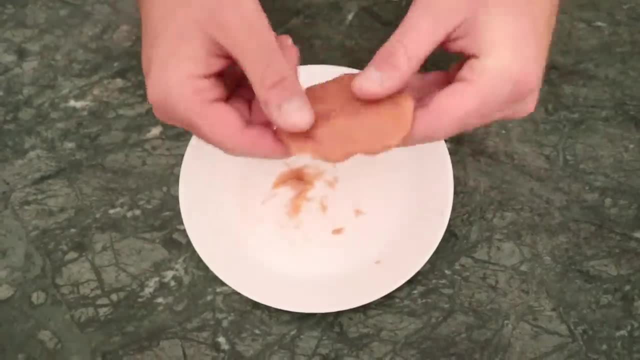 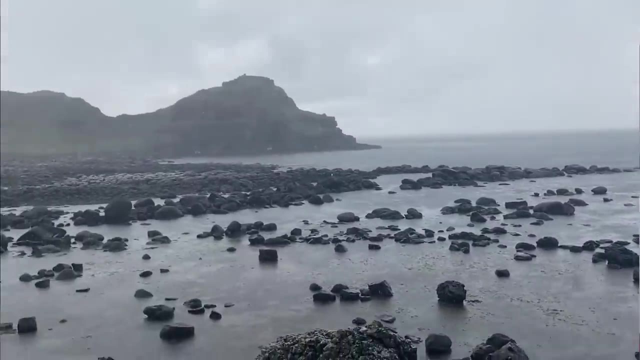 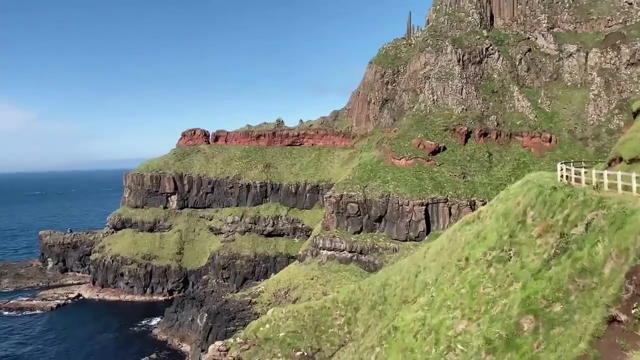 Then, when they cool down again, they harden to form igneous rock. Then, once again, over a super long time, this igneous rock is chipped away by the wind and rain. These tiny pieces of rocks and dirt are then once again carried away by the water, from streams to rivers, to lakes and oceans, where they sink down to the bottom. 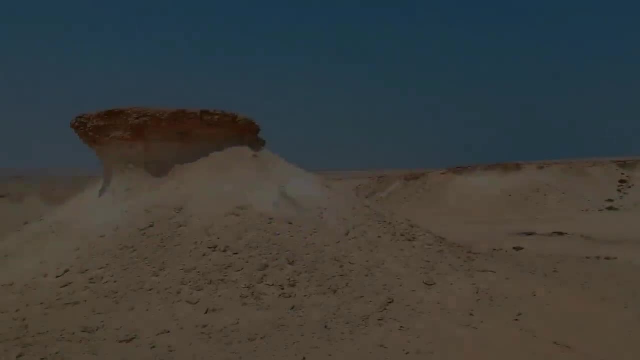 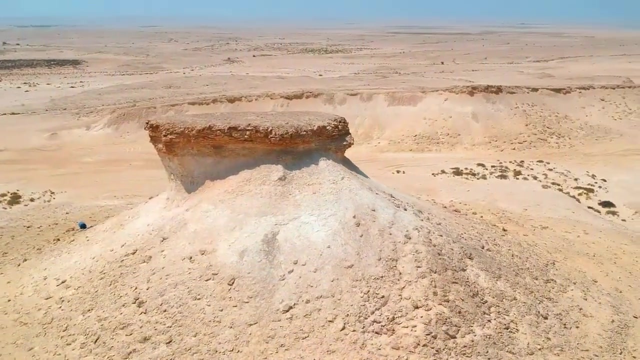 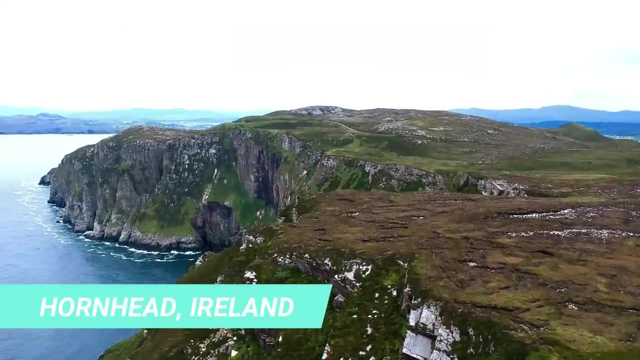 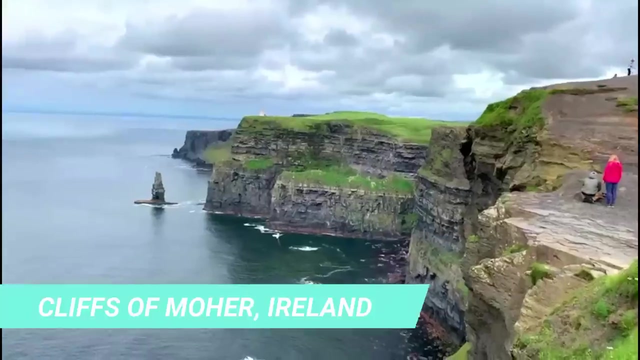 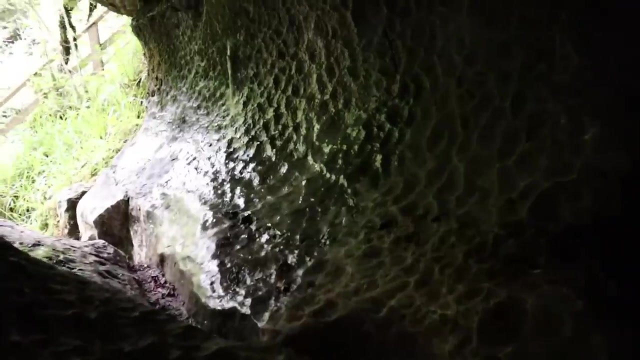 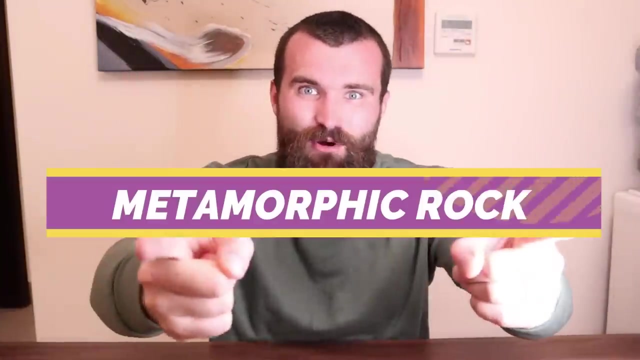 Let's check out some incredible sedimentary rock formations. Let's check out some incredible sedimentary rock formations, And the next type of rock we're going to learn about is metamorphic rock. Sometimes these layers of rocks and dirt deep underground become close to molten hot magma. 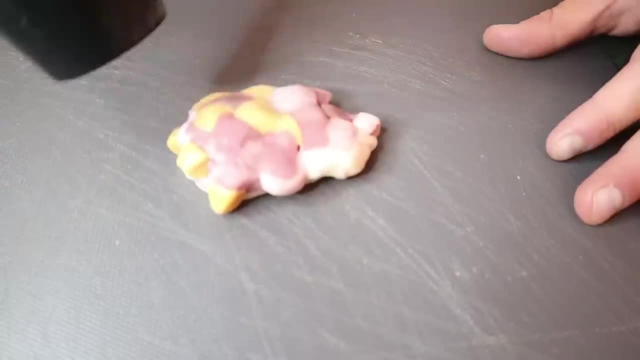 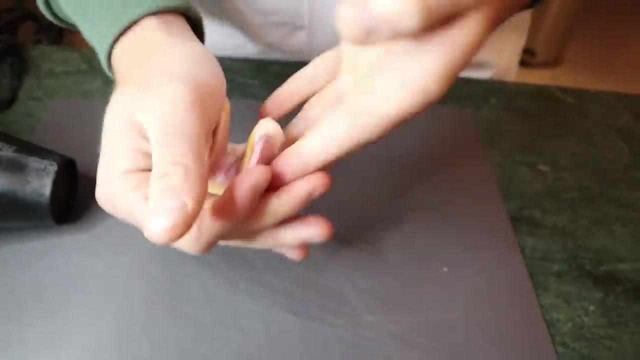 To add a little bit of heat to this rock, I'm going to use a hair dryer. The heat of the magma, combined with the huge pressure of all of the layers of rocks above, can cause the rocks at the bottom to be chemically changed into metamorphic rock. 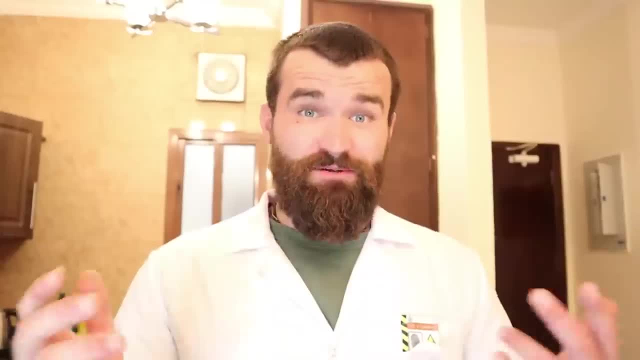 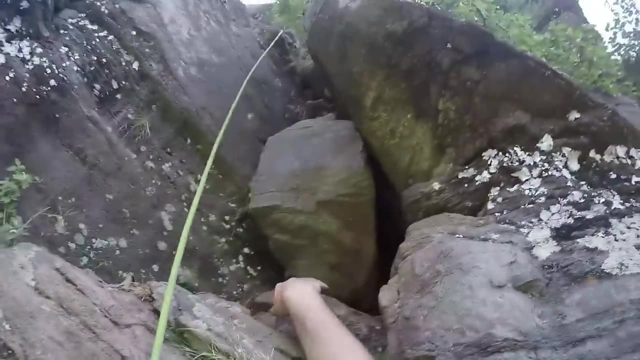 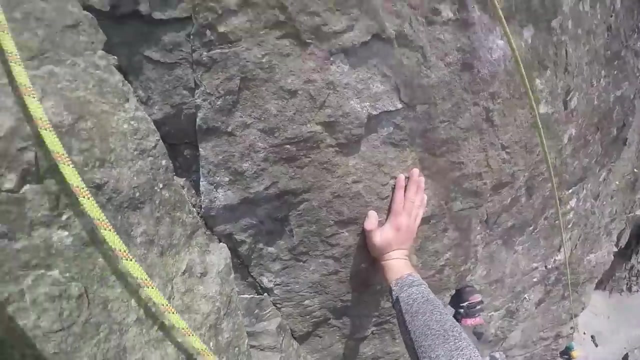 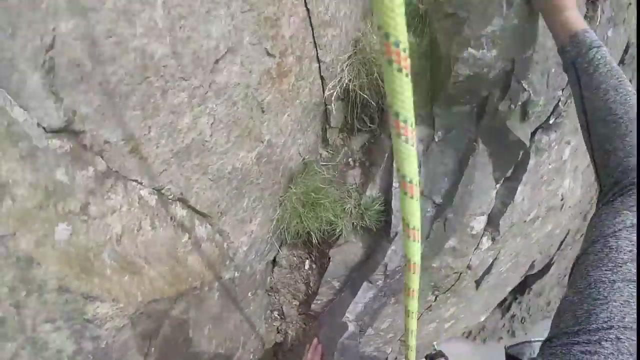 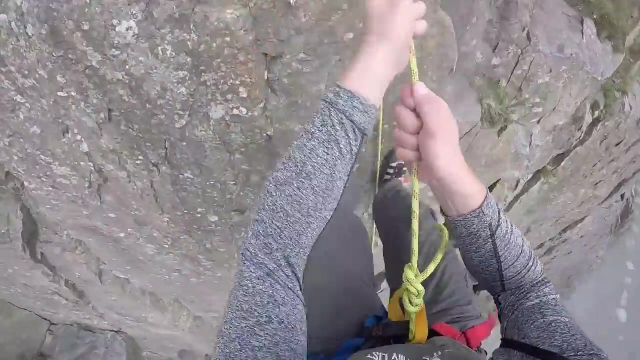 But this also takes a super long time. Here's some footage of me climbing on metamorphic rock on a mountaineering course in India: Sea rock- Sea rock. The next type of rock we're going to learn about is igneous rock. 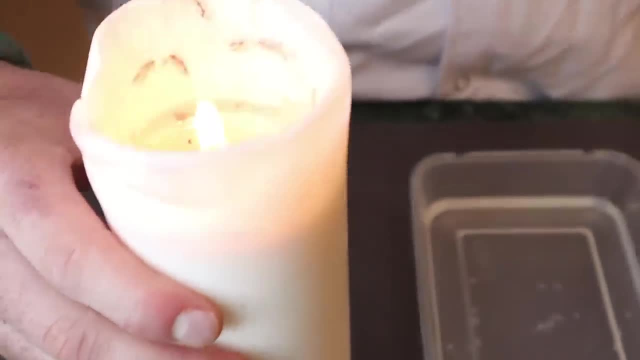 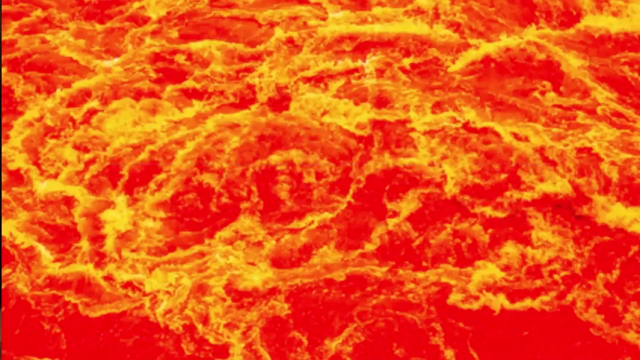 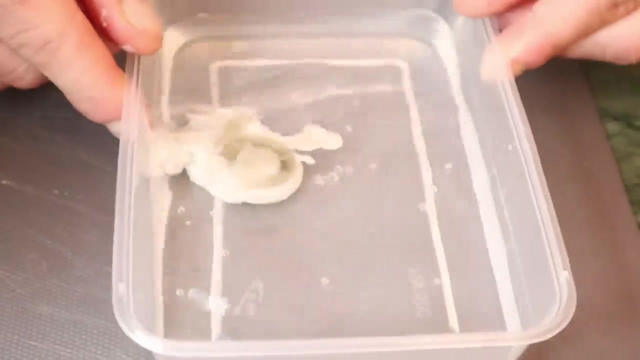 Igneous rock is formed when rocks become so hot that they melt and turn to liquid. We call them molten rocks. Molten rock that is underground is called magma, And molten rock that comes out of the ground is called lava. When the magma or lava cools down again, it hardens and forms igneous rock. 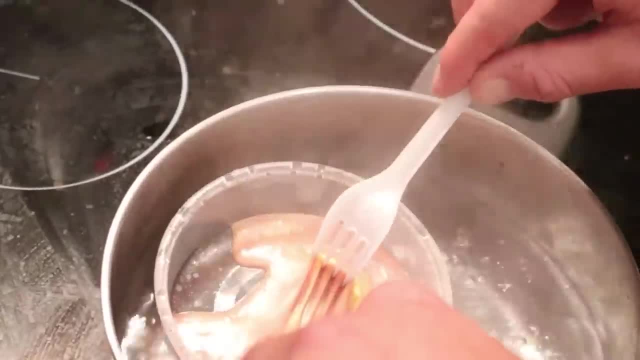 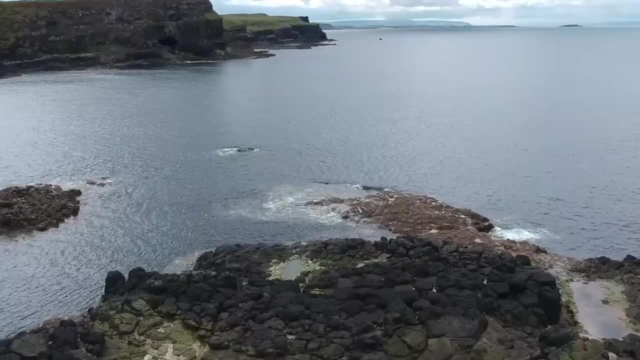 Take a look at my starburst. When I heat them, they begin to melt and form molten rock. Then, when they cool down again, they harden to form igneous rock. Then, once again, over a super long time, this igneous rock is chipped away by the wind and rain. 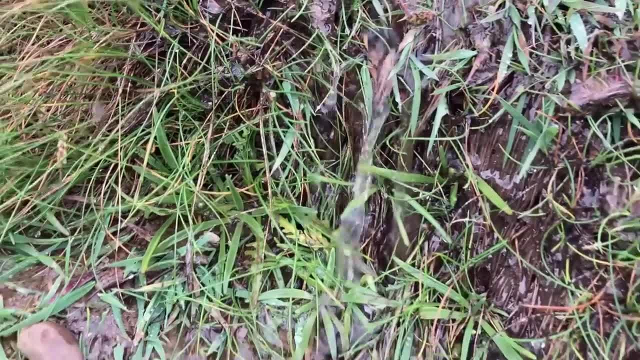 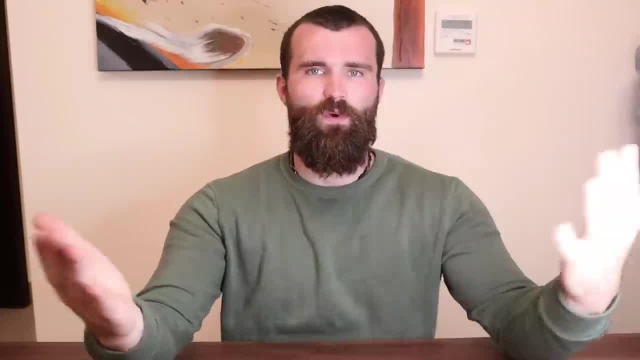 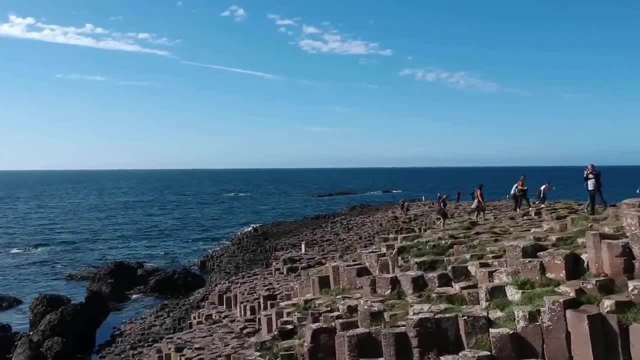 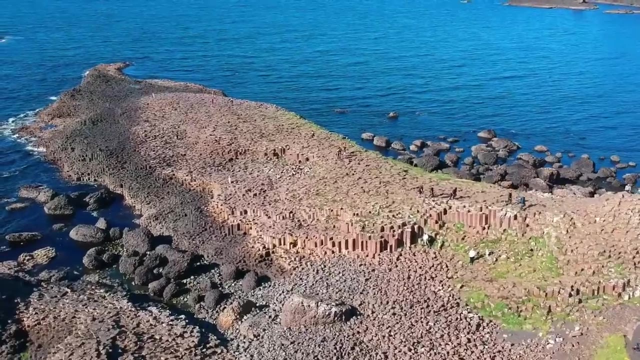 These tiny pieces of rocks and dirt are then once again carried away by the water, from streams to rivers, to lakes and oceans, where they sink down to the bottom, And the cycle begins all over again. We call this the rock cycle. Hi guys, I'm here at the Giant's Causeway.